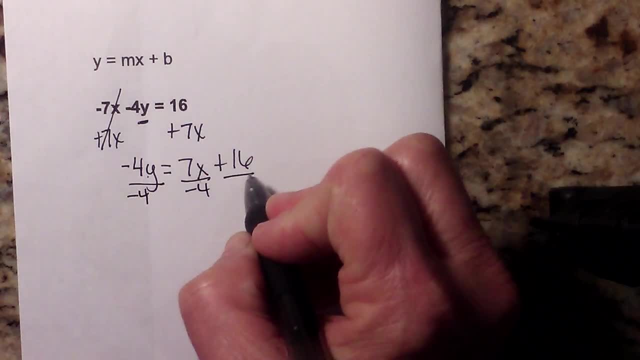 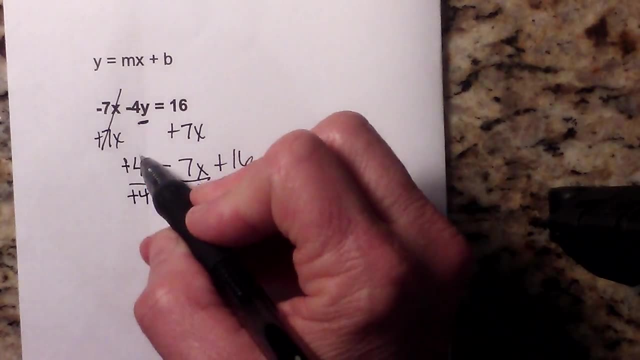 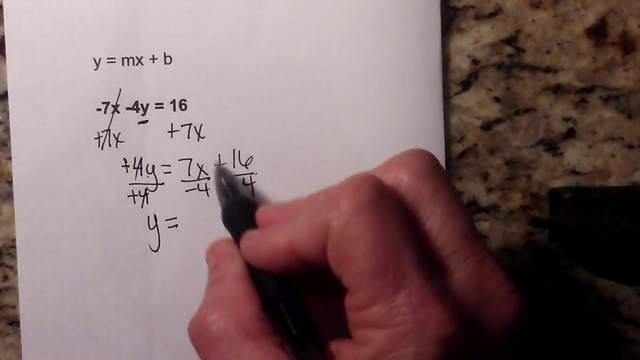 So we're going to divide, to undo that. So we're going to divide every single term by negative 4.. Well, what happens is this term negative 4y. all the 4 cancels out and the negatives cancel out, And we're just left with y. Okay, this term is negative 7, fourths x and 16 divided by negative 4. 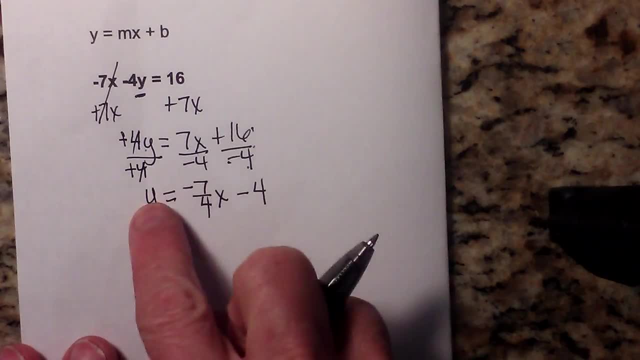 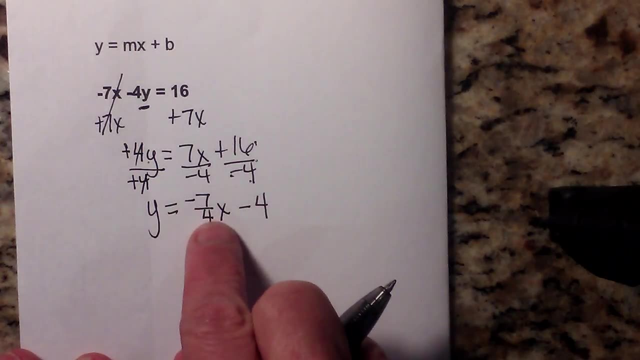 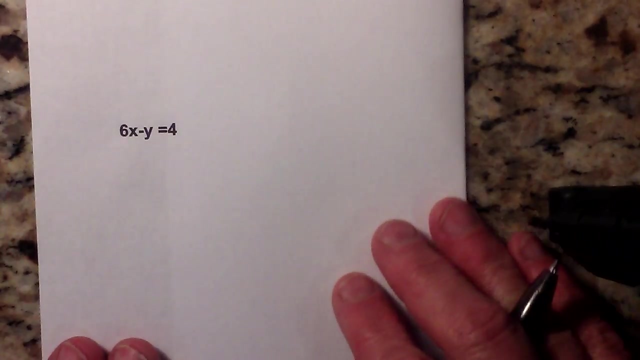 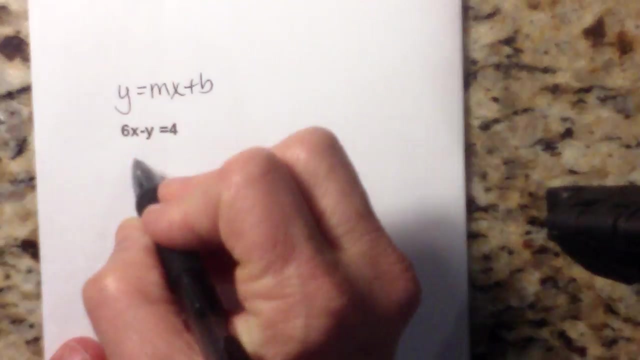 is negative 4.. So now we have the equation in the form y equals mx plus b, where the slope is negative 7 fourths and the y intercept is negative 4.. Okay, so let's try a second one. Again, we're trying to change it to the form y equals mx plus b. So we are trying to solve for y. 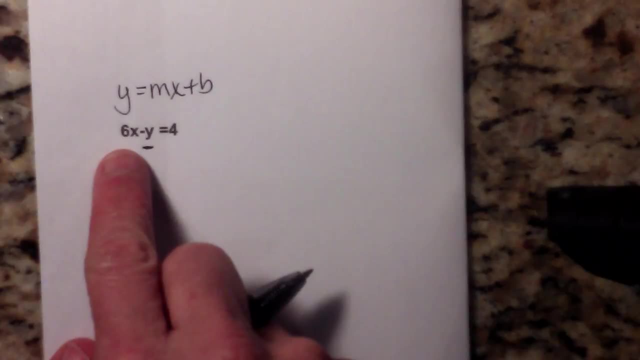 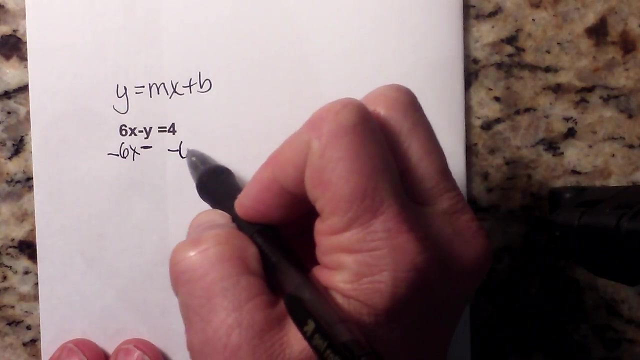 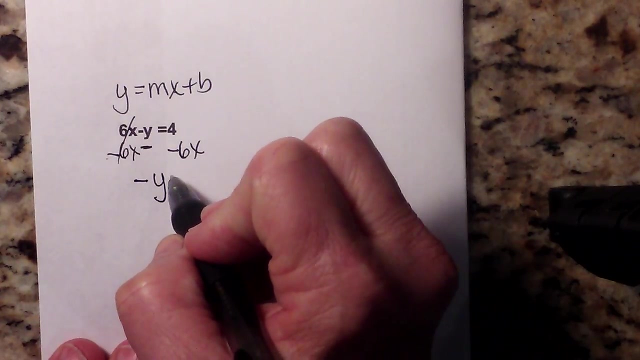 So we need to get the y by itself. So what do we need to move? We need to move this 6x. Okay, it's a positive 6x, So I'm going to subtract it from both sides. Okay, 6x minus 6x, that cancels. I'm going to bring down a negative. y is equal to and again, I'm going. 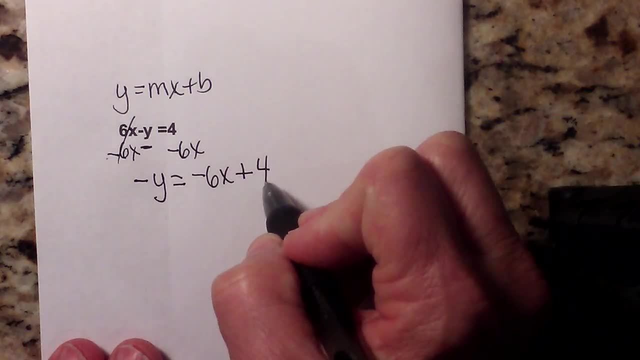 to put my negative 6x forward. So I'm going to subtract it from both sides. So I'm going to bring down a negative: y is equal to, and again I'm going to put my negative 6x forward And then my constant: a positive 4. last Now is the y by itself? No, it's not. We have a negative. 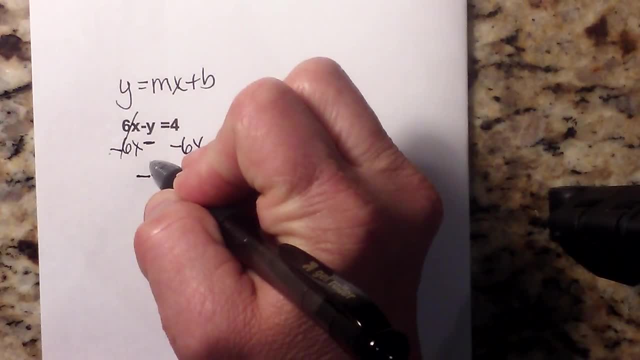 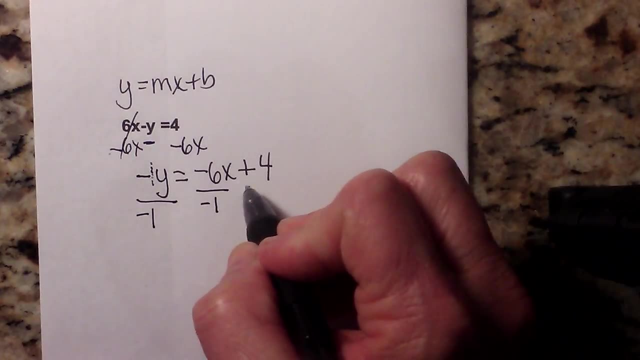 coefficient. Well, that's actually a negative 1.. So I'm going to draw a little 1 here. Okay, we need to get rid of the negative 1.. So we're going to divide every term by negative 1.. So this, these: 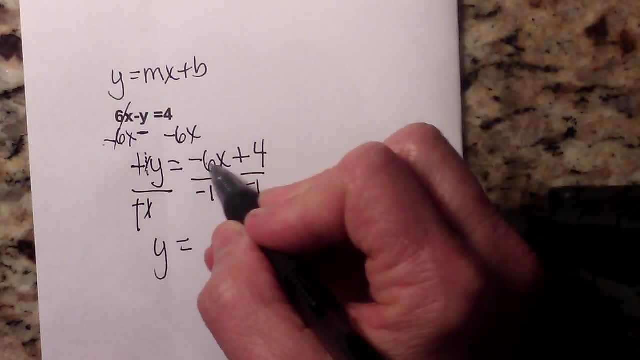 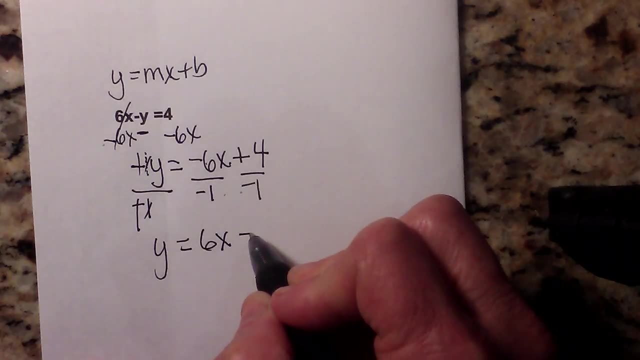 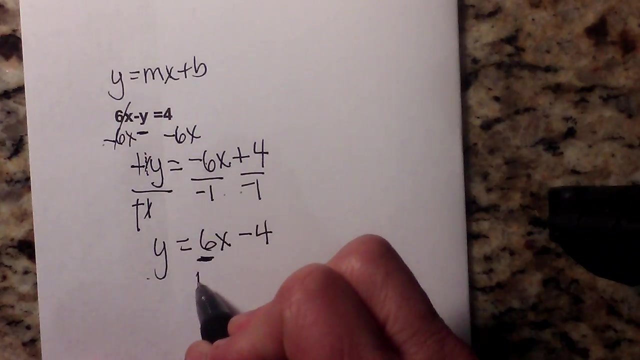 cancel and I'm just left with y Negative 6x. divided by negative, 1 is positive 6x and 4. Divided by negative, 1 is negative, 4.. And here we have the equation in slope intercept form, where the slope is 6 and the y intercept b is negative, 4.. Hope this video is helpful. 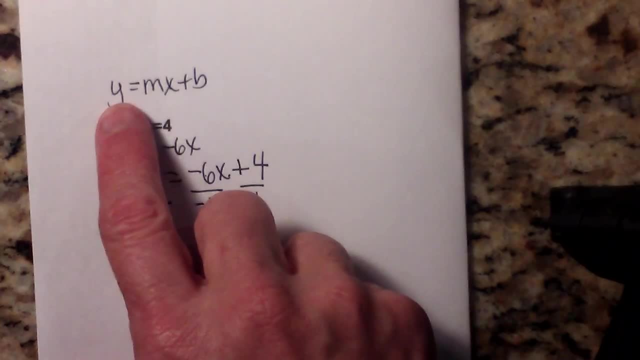 in learning how to change forms to slope intercept form.